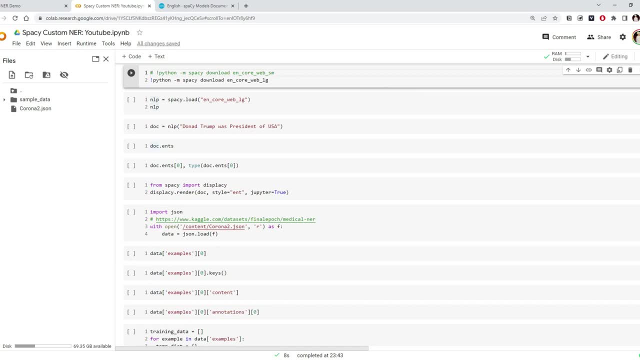 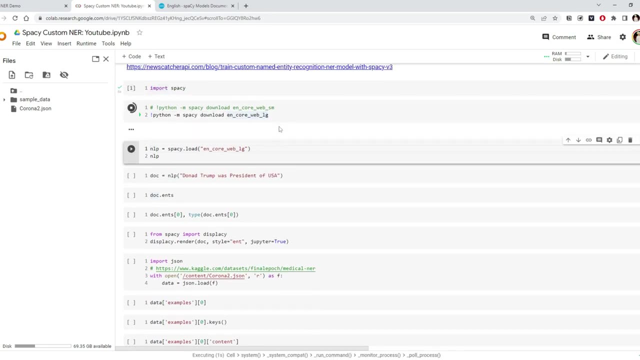 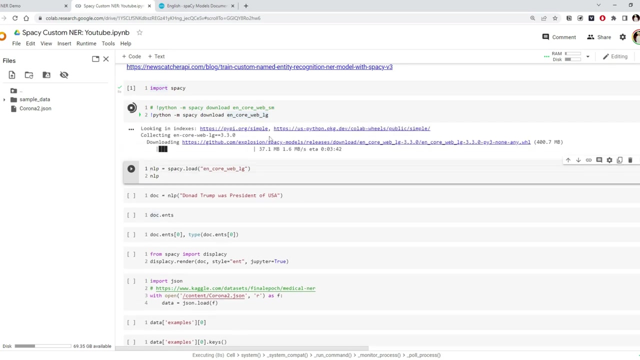 collab notebook. we have imported spaCy and then we can use spaCy download command to download this particular model that we are interested. it might take some time, like maybe 40 seconds to one minute, so seems to be. it is 400 MB model and once we download the model we can use this spaCy. 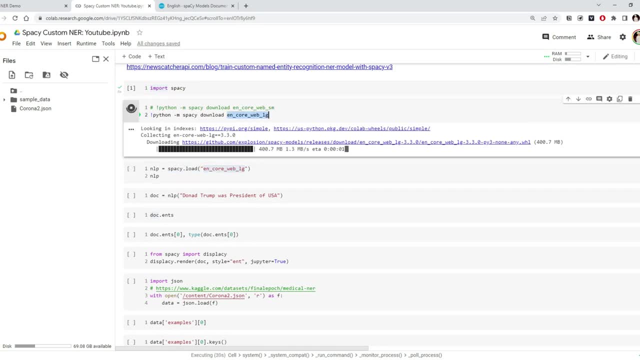 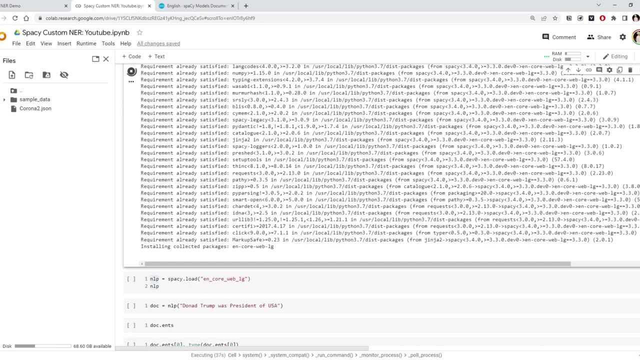 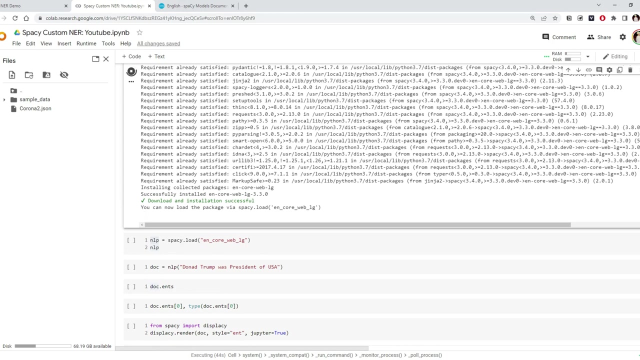 dot load method and specify the name of the model without just be downloaded, and the model will be loaded in this variable. we normally call it nlp variable. currently it has downloaded, now it is installing. okay, it has installed successfully. now we can see we can load that model using this. 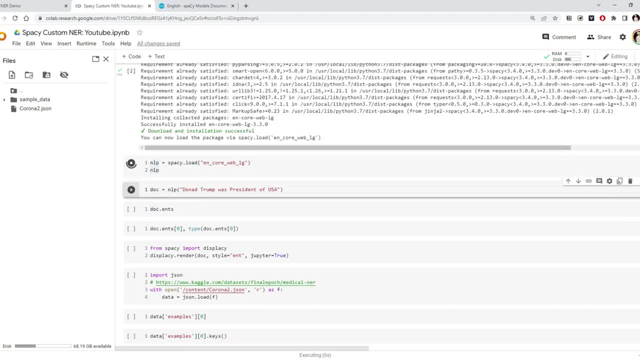 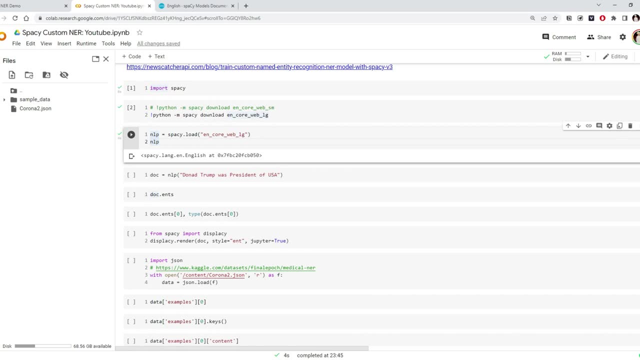 spacey dot load method. it's loading meanwhile. i will just clear this output here. yeah, now it is loaded in this nlp variable and we can see it is of a type spaty language, english instance. once we have a spacey language model, we can pass any document or a text into it. 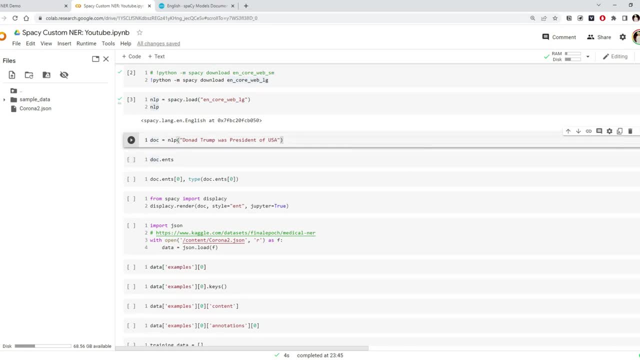 and it will create a document object. so let's run this statement and we can see it is a type of the dot. first, we will see what is inside the talk. so doc object looks like something like this: so you can see what is inside the doc. so the document object looks like: 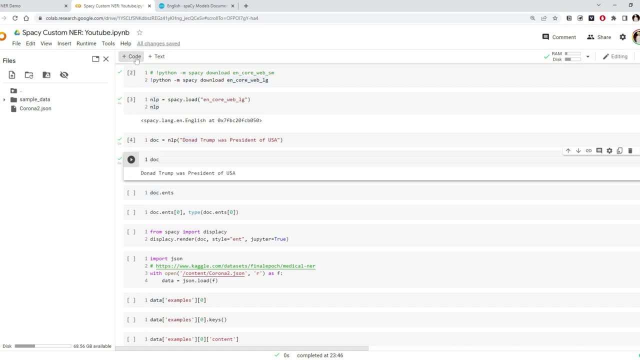 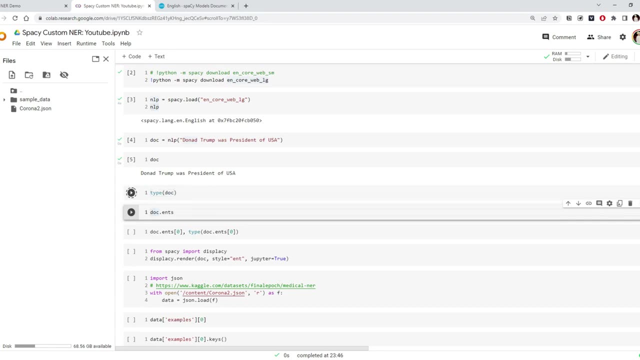 same what we have passed, similar to the text, but it has a different properties now because it is processed by the specie language model and we can also check the type of the doc variable. so type of the doc variable is the type doc. so specie has a specific variable. 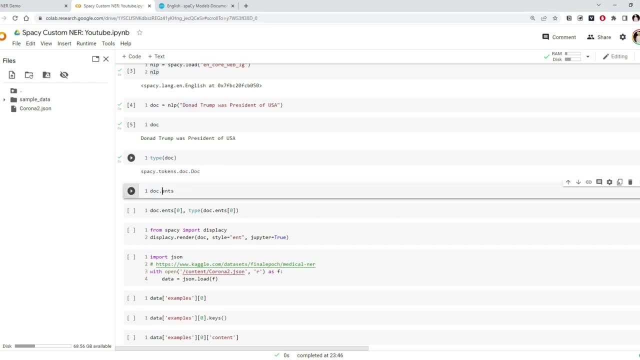 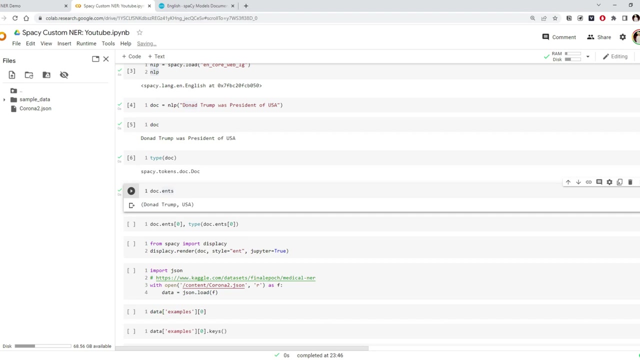 called a doc and this doc object has a property called entities or entities. and this is where all the extracted entities, the name entities, we can find out. so if i click we can see from the above text it has found out two entities, donald trump and usa. 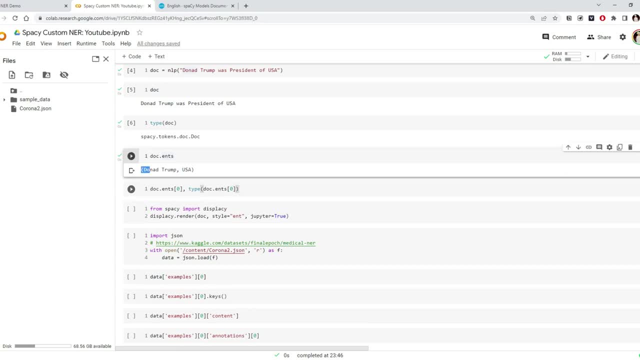 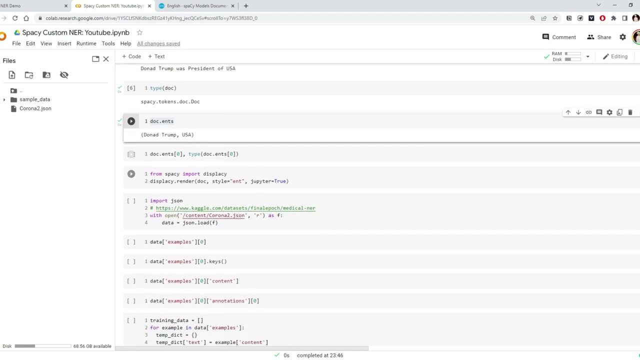 and we could, which we can first of all see. even the entity is of some type, specific. each entity in these entities is of subspecific type. we can also see dot, dot. entities will be the list of entity and each entity has some type. let's visualize what is the type of this, each entity. 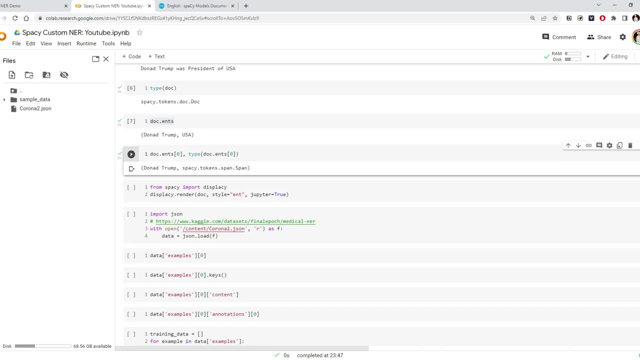 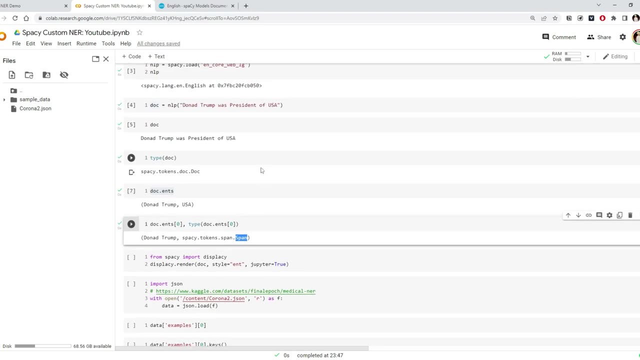 okay, so here is the entity donald trump, and we can see thus: this is a specific type of the specie object, called a span object. now, this information is important, that how did we pass information, let's say text, to the nlp object and then we got a type of doc, object of type doc, and then doc. 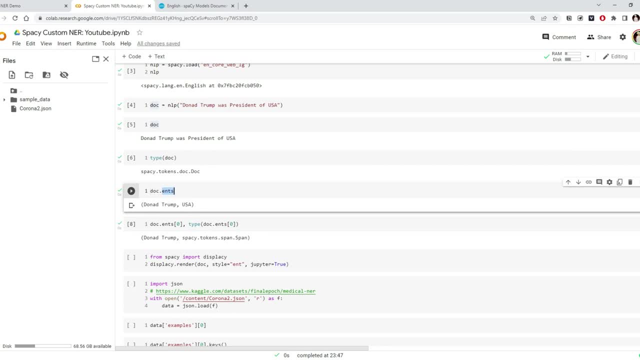 stores all the entities inside this entities variable and each entity in this entire and each entity inside this entities variable is of type span because when we going to train spacey model for a custom name entity recognition, we have to create our training data in the same format. we have to take each training example like this: 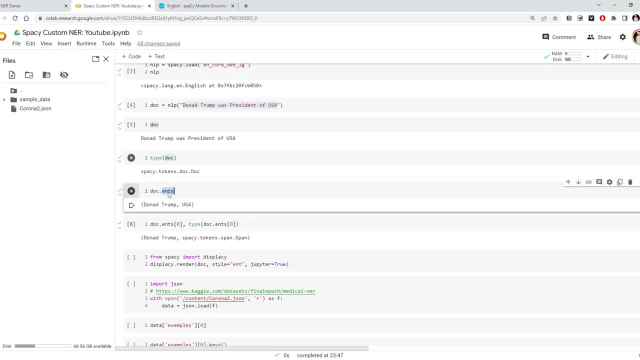 create a doc object and then add entities available in our training example as a list of span object and then, once we train the spacey, spacey will be able to predict the same way custom entity, just like it is able to predict the donald trump and the usa as an entity, and spacey has some visualization. 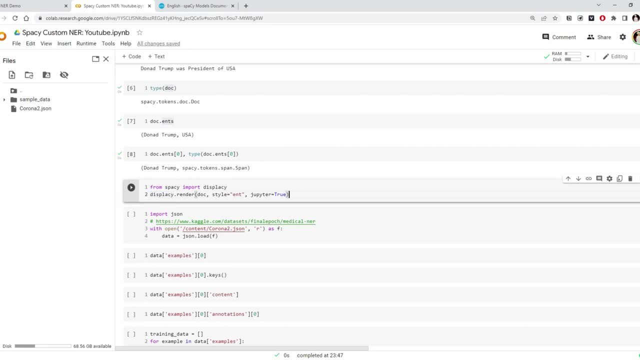 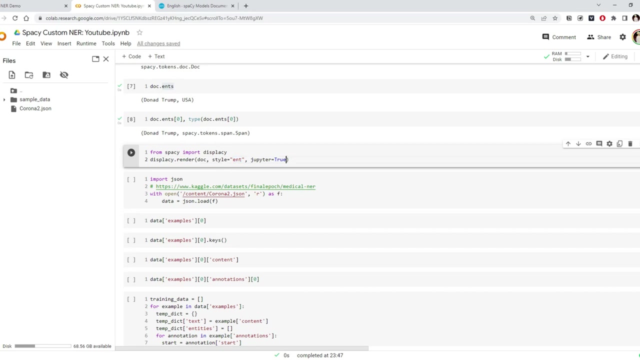 module where we can visualize the entities it has predicted. so we use displacing and it has a rendered method which take the dark objects processed by the spacey module. and then we have to use style and we are want to visualize entities and since we are in the collab notebook, we call 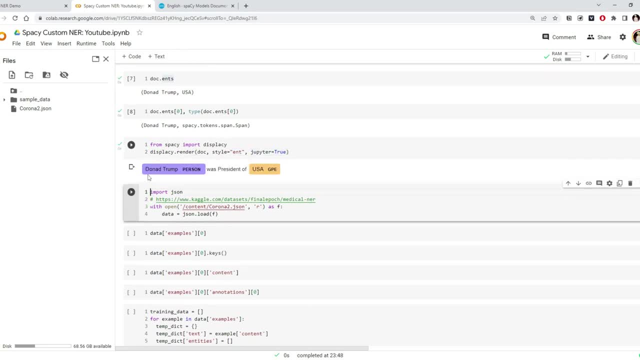 jupiter as a true and then it will visualize. now we can see it has identified donald trump as a type of person and usa as a gpe. here gp is geopolitical entity, so it is able to identify a specific or generic entities like person, place, organization. but our goal is to build. 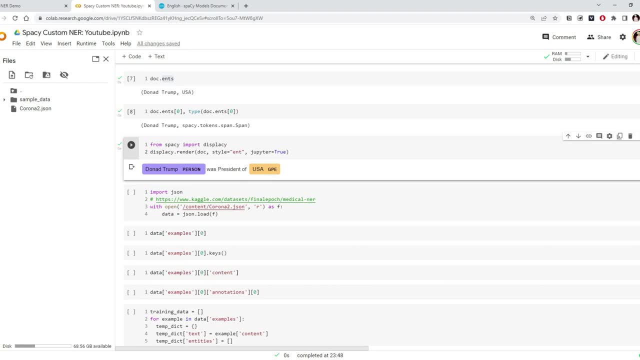 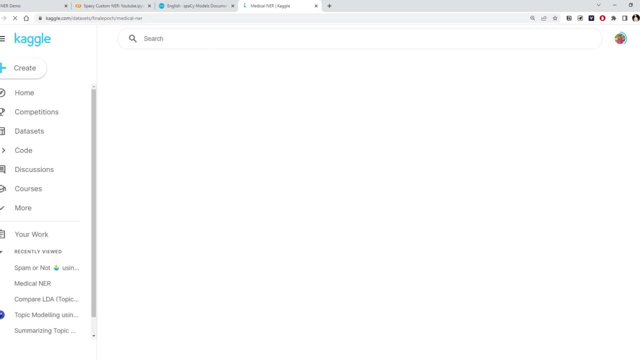 spacey model which will identify entities of our interest. so we have some medical data. i took this data from the kegel and we want to use this medical ner data, which is already tagged for the medical entities, so let's go to there. yeah, so we do have this, you know data. 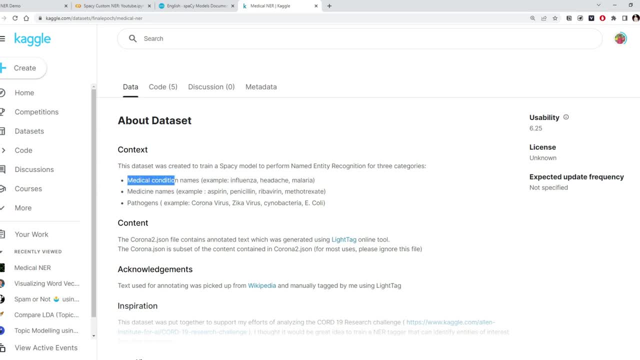 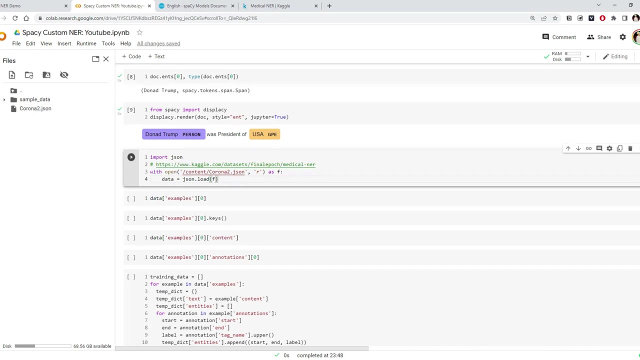 which has some type of entities, like it has some medical condition, it has some medicine named pathogens and we want to identify those entities. so let's go back to our and load the data. so i have already downloaded that particular data set, which is the medical ner: medical name, entity recognition. 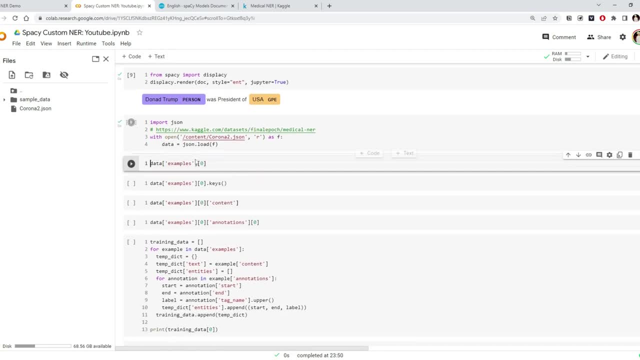 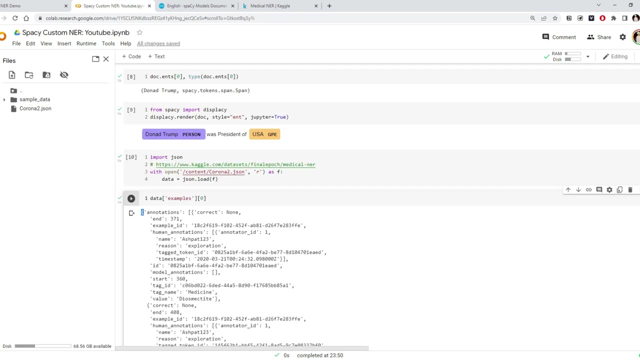 let's load that data set and the data set gets loaded into the data example. so here is what all examples. we have training examples. we can look at the training example. okay, it seems to be, there is a lot of things, but we can see each training example. 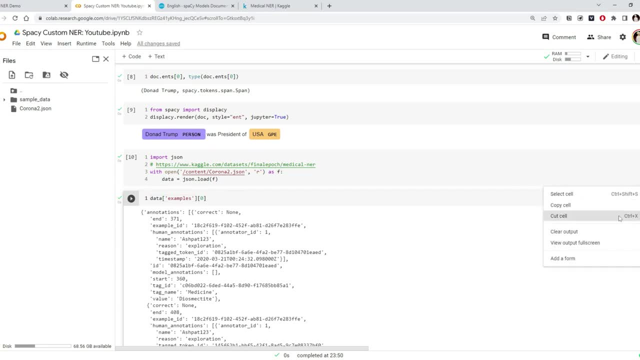 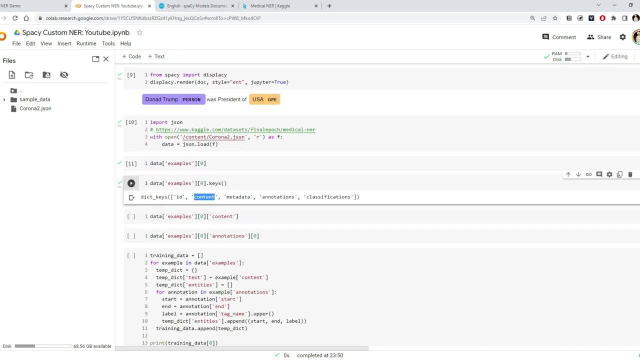 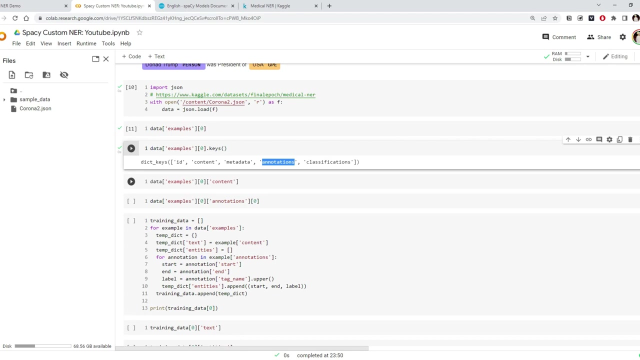 is actually one dictionary, so we can look at what are the keys of that dictionary first. so let's look at what are the keys of the dictionary. so the dictionary has content, annotations, metadata and classification. we are interested in content and annotations, so let's look at, for a first example, what does content field has. 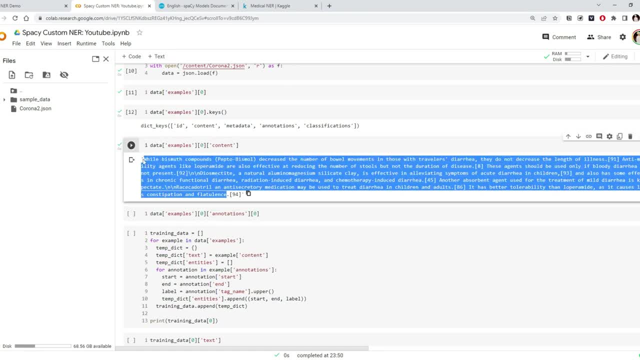 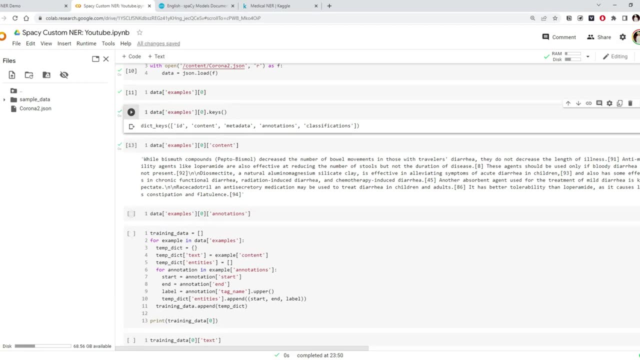 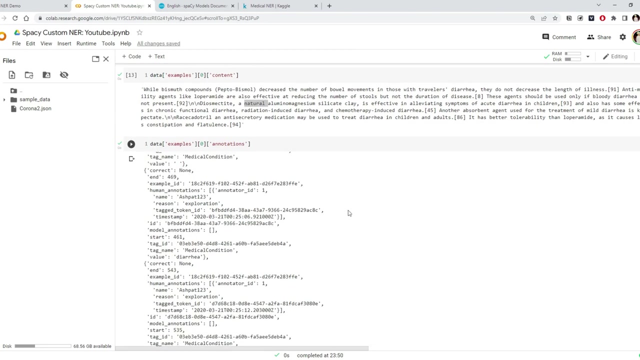 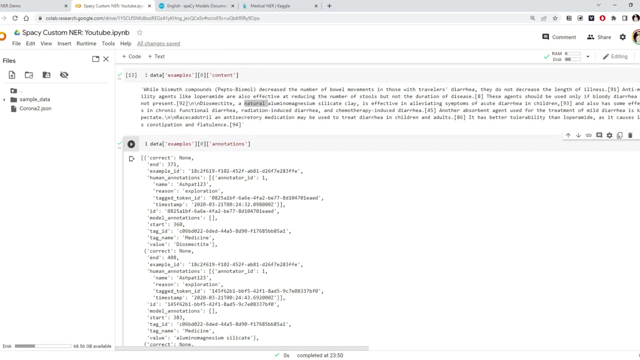 so content is nothing but some medical text. and then, for the same example, we can also see the annotations field, which will be having all the entities found in this text, and we can see it has many entities. the first example that we are checking has a multiple entities because we have a list of entities. so let's look at any particular entity and see. 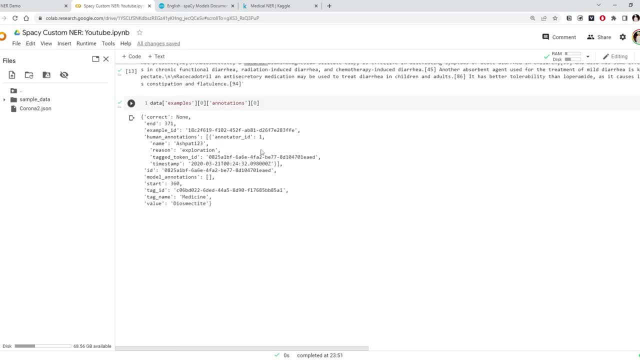 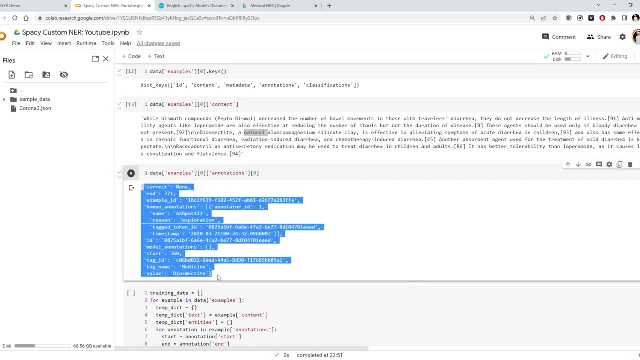 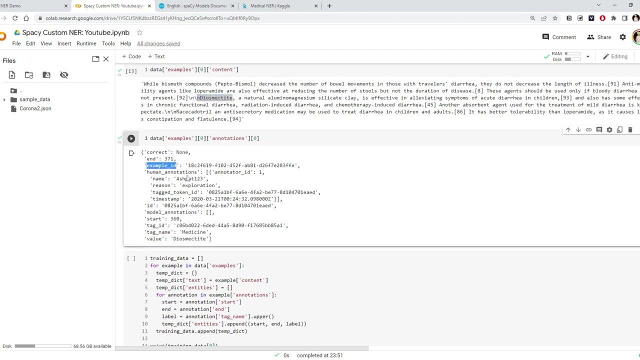 what all field that entity annotation has. so the kaggle data contains this annotated information for each entity present in each example and we can look at. we have example id. we also have the human annotator who has annotated this thing. but we are interested in what is the tag name, which is the type of the name entity. so 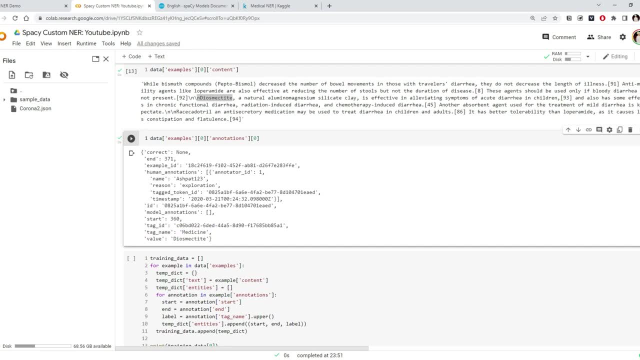 this particular entity is of type medicine and where does the tag name come from? so this particular entity is of type medicine. it is located. we can see it's a start index in this text and the end index in this text. so the entity medicine of type medicine is located at the 360 index in this text and which is ending: 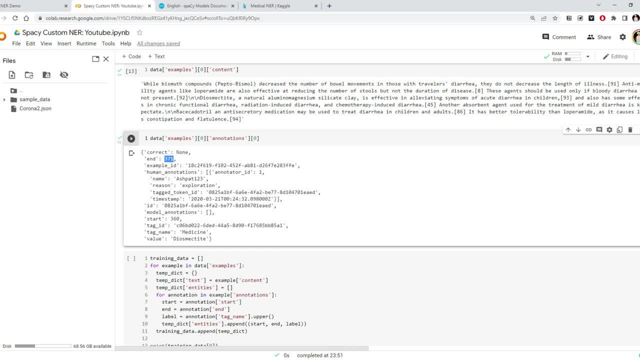 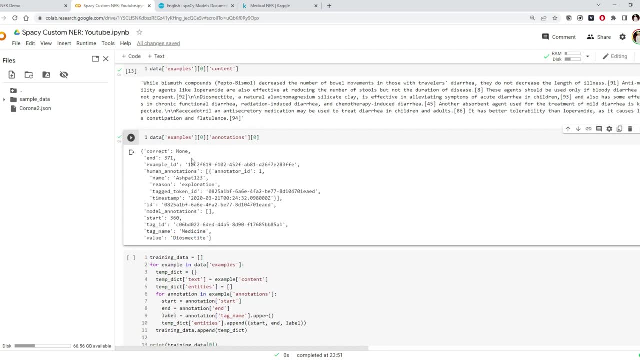 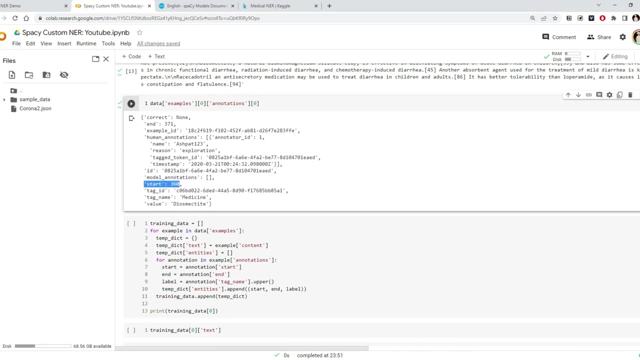 at 371. so whatever between 360 and 371 is of type medicine and actually that text is this particular value. okay, so we saw what is there, but we are only interested in three things. we are interested in which is the tag name: where does it start and where does it end? so let's. 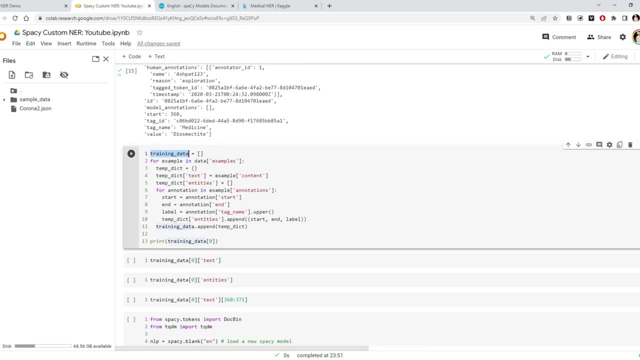 take this few things of our interest. so we will create a new variable or the list of training data. here we will iterate through our data examples what we just loaded from the Kaggle, and then from each example we will take the content field, that is where the text is located, and then we will also take the 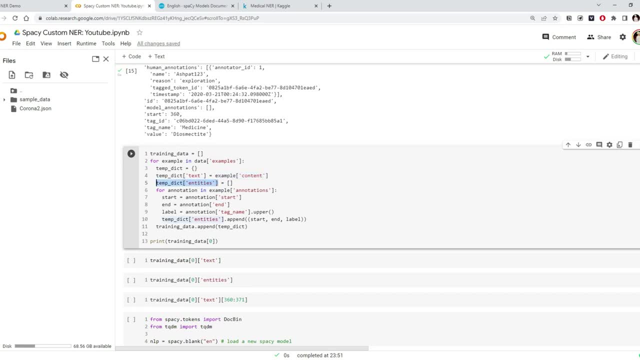 entities field. to get that entities field, each example has the annotation. that's what we look at here. so we will iterate through those annotations and we will only take annotations. start and end the tag name, as we discussed, and then for each example we are putting all that information in a temporal dictionary. 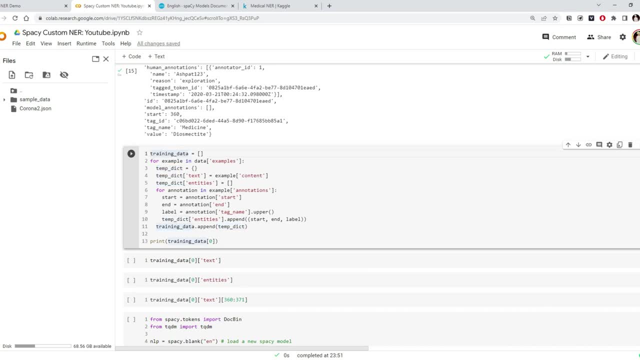 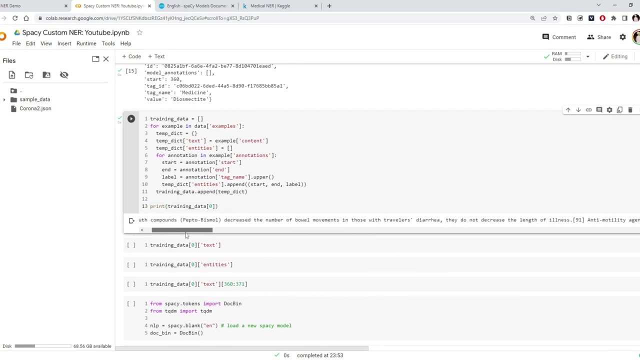 and then eventually we are appending that dictionary to our training data. so our training data is nothing but the list of dictionaries, where each dictionary is holding our one example, and we can look at what is the first example we got after preprocess. so example as a statement field, and then it has entities field, and entities is again a list of entities in. 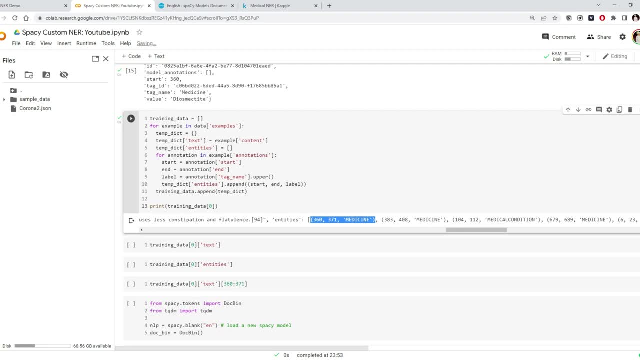 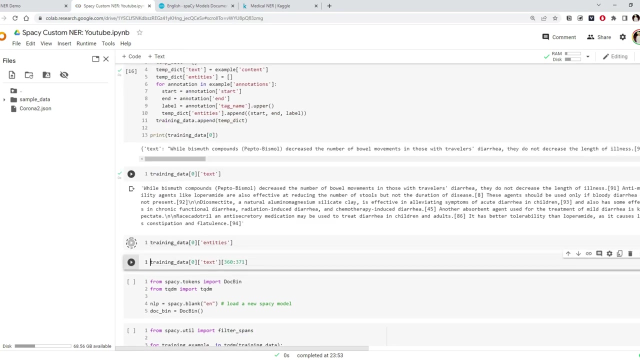 that text and each entity. you can see we have three things a tuple here: the starting index, ending index and the type of the entities, what we have inside that particular text. we can see it better way here. what is the text? what is the entities here? yeah, we can see we have many entities and we can see the first. 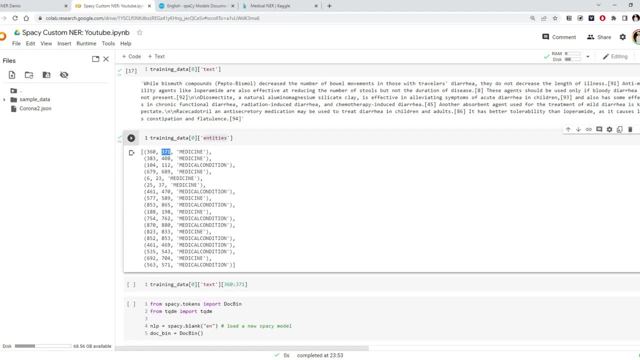 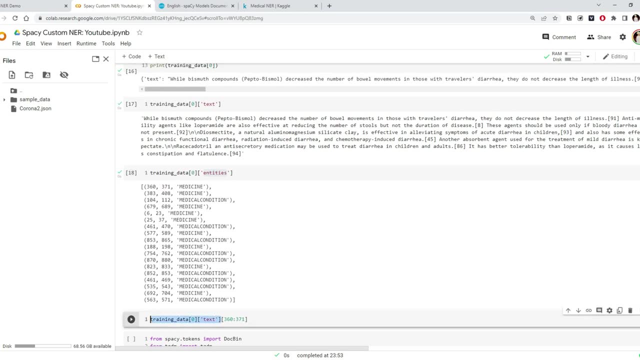 entity is located between 360 and 371, we can also see what is the value of that particular entity. so let's take the first example text field and just see- since it is a string we can- and index it using we can see what from 360 to 372. 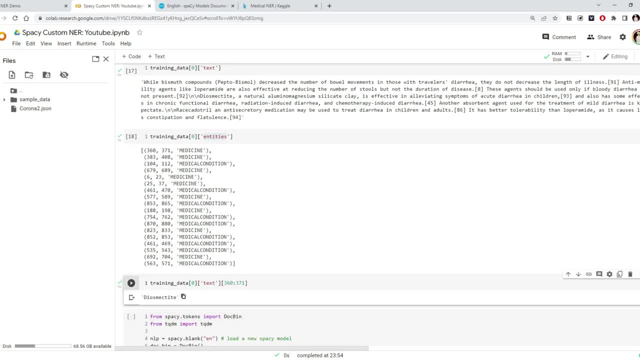 what is located? yeah, so this is the value located inside the string at the index 360 to 372, which is of type medicine, and that's what we want to teach our specie model that how does the medicine type look like? and similarly we have medical. 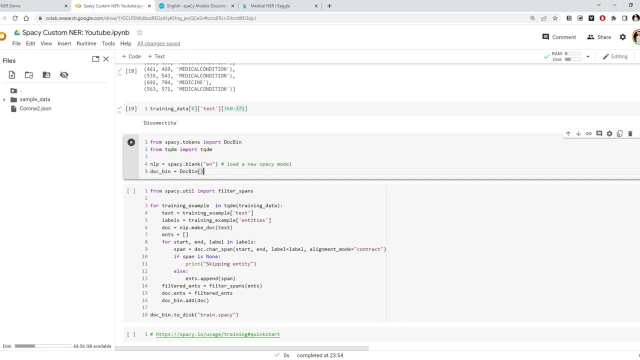 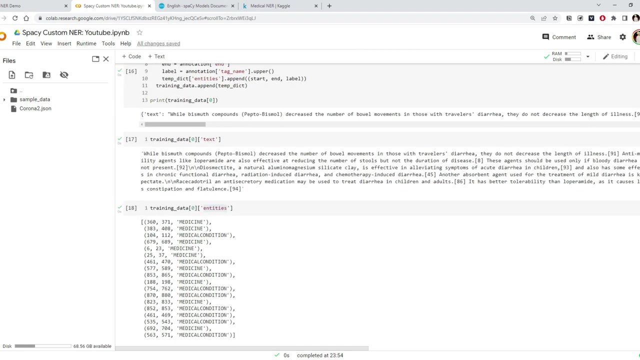 condition and the other types also. to train a specie model, specie required training data to be in a particular format: specie advice. the training data should be of a type dog bean and which will be saved as a dot specie format. and do you remember earlier when I talked about how does specie does prediction on? 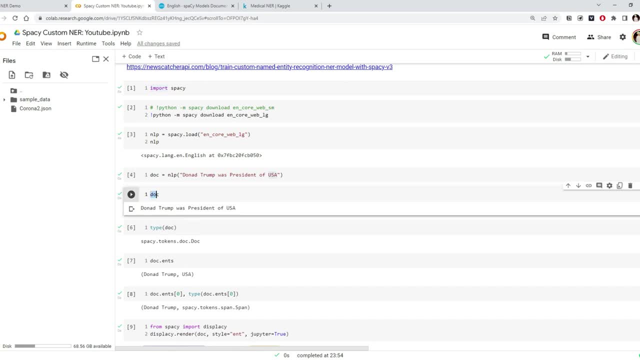 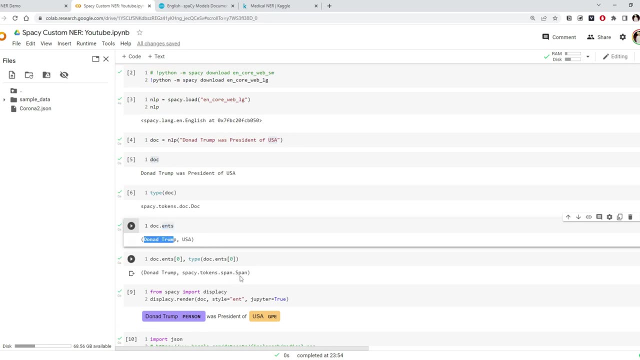 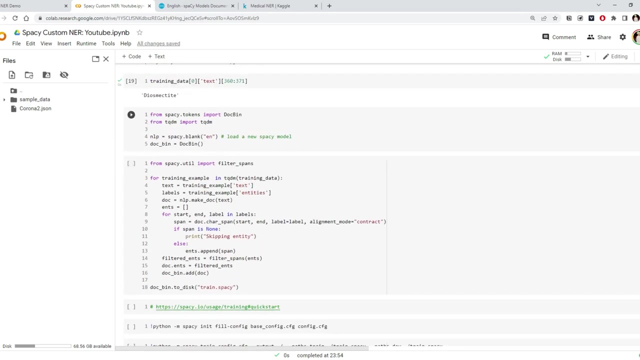 data. when we pass the text, it has a dog object and the dog object has entities filled, and then each entity is nothing but actually a span object. and we have to do the same thing. we have to convert our training data in the document- entities and the span object. so let's go back here. so the first thing we will 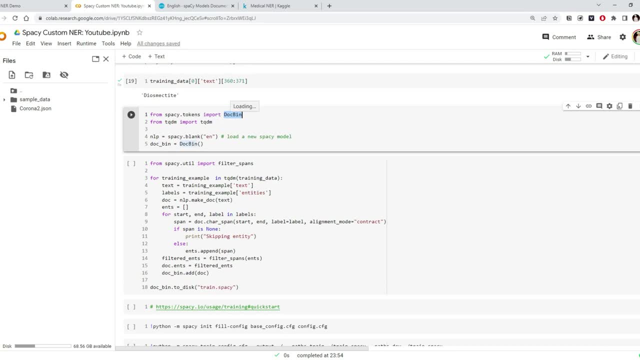 import a dog bean object. this is the object where we going to a paid or all documents that we going to create, and we will use the blank specie model here and then we will also use some utility, a filter span. utility comes. we will see what it is. now let's iterate through our training data, what we have currently and 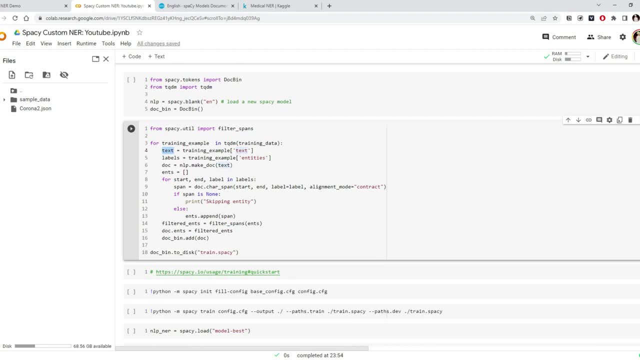 for each example, we took our text field and then we take our all entities and we call them as the labels. as I mentioned, we have to create a document object for each example. so, using the NLP language object, it has a method- make talk- which will take our text field for. 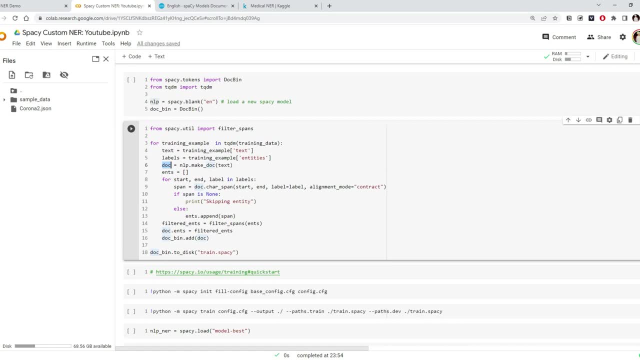 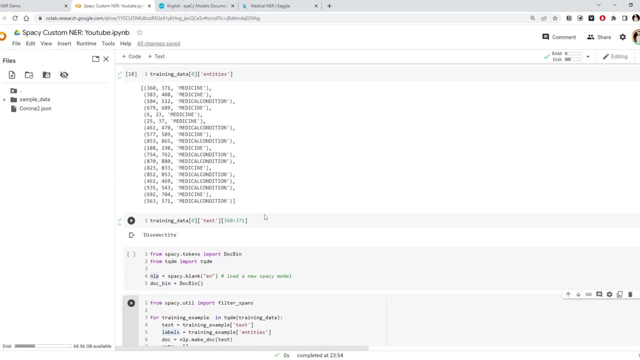 that particular example. now we got a dog object. now we want to append entities to this dog object. so first we will collect our entities available inside this label filter, so we'll iterate through our labels and we know each of our entity label or entity annotation has three things: start, end and the type of the entities. right, so 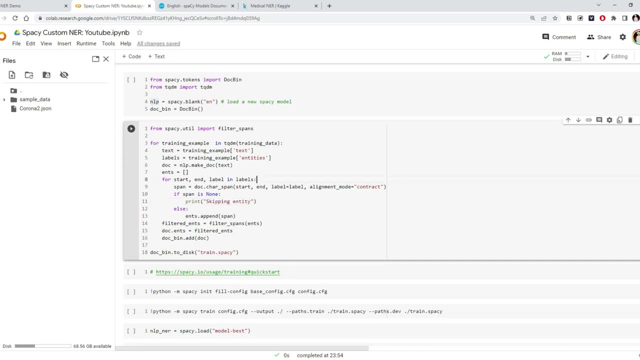 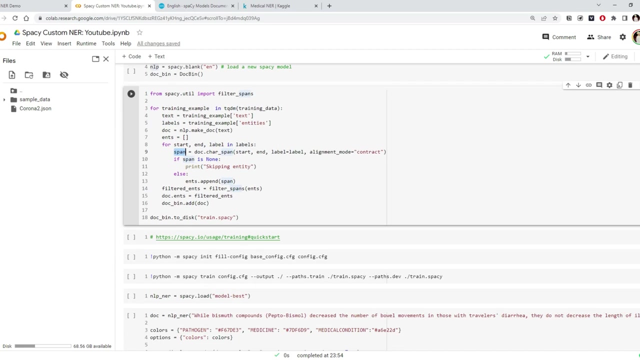 this is where we're going to create for each entity a span object. we can create using the method dot, dot, character span. we can create that span object giving this three information: starting, ending and the label. and once we have a span object, we check some sanity, check whether the span is none. if it is none, we will skip that. 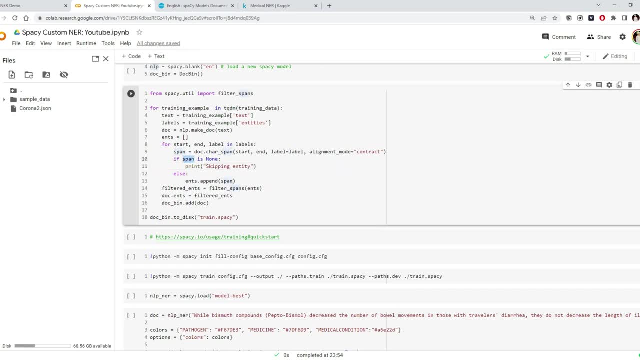 particular annotation and if it is a valid span, we're going to append in our list of entities. and once we have all the entities for that example- training example- we will pass those entities to the filter span. so, filter span, make sure we don't have any duplicate. 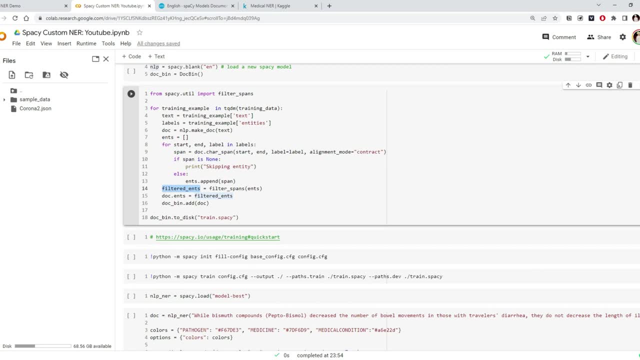 entities and it checks for other sanity checks and once we get those filtered entities, we want to put it as a part of dogentities variable and we will simply put those entities inside this dogentities. and this is where we created our first document, using our first example, and 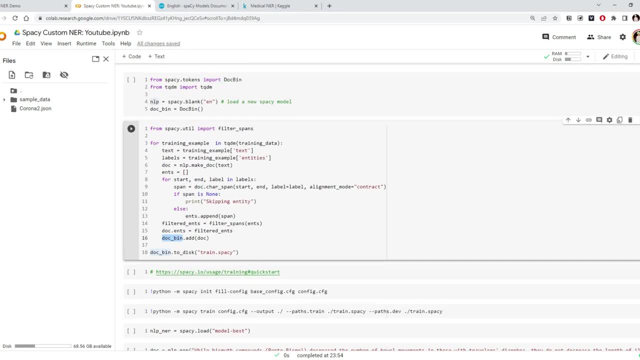 then we will append the document to the document object that we created on the top, and once we process all such examples, we will have a dog bin object which is nothing but the list of document that we created, and we will save it to the disk. so let's run this set. 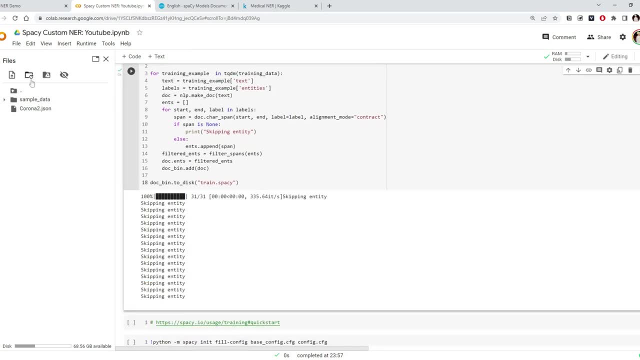 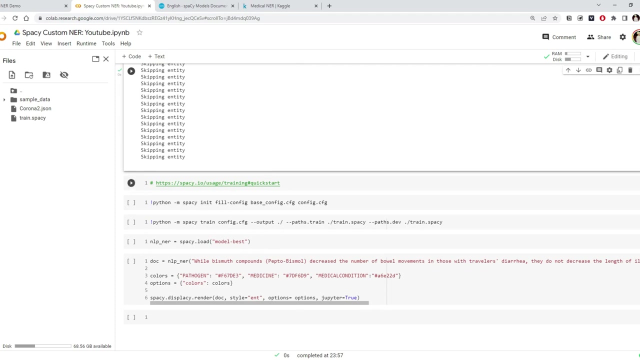 okay, it also skips some of the entities and it should now, if I refresh here, we should see we can see the trainspec file cup. now we have a data which is required by the specie format. next thing: before we start spacing, model training specie require a config file and if you go to this URL, 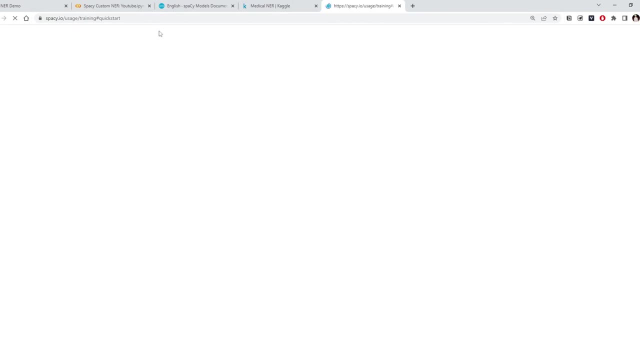 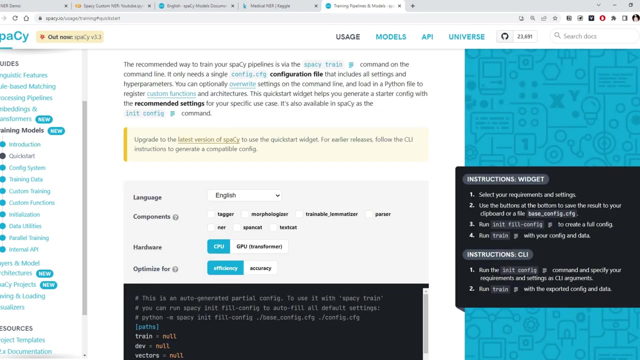 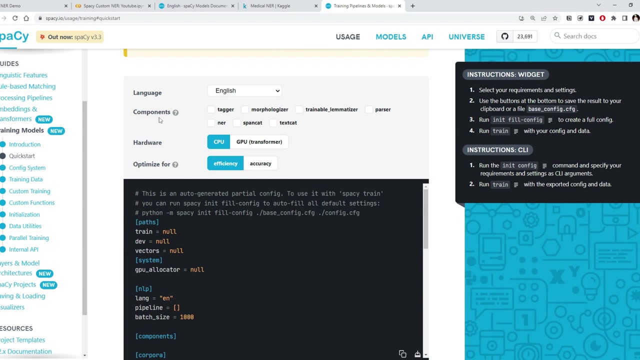 where specie explains or specie helps you to create that config file. okay, if I go to this quick start URL, here is the UI to create your config file. so it suggests which language we want to build- so we want to use the English language- and what components we are. 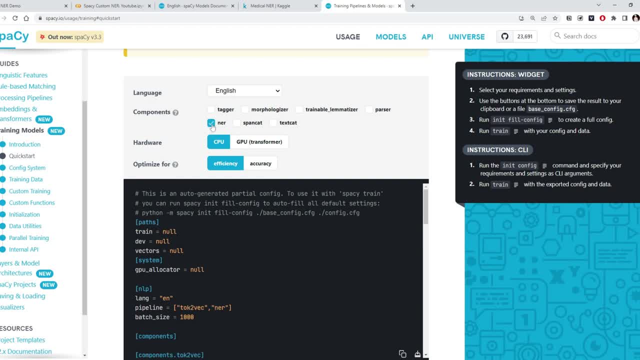 interested in. we are interested in the NE and the name entity recognition here, whether we want to run it on GPU or CPU. currently we are interested on CPU. then we have choice whether we want efficiency or accuracy. efficiency, the models will be the smaller. accurate model will be the faster, oh sorry, the. 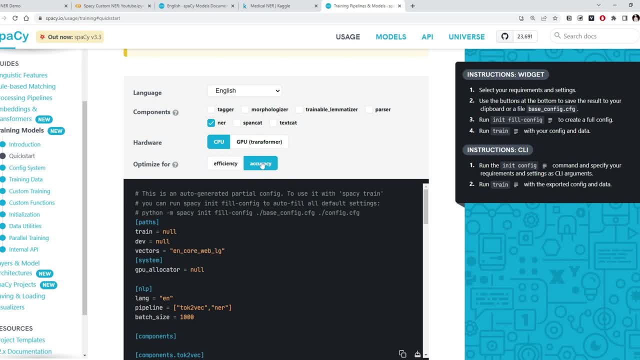 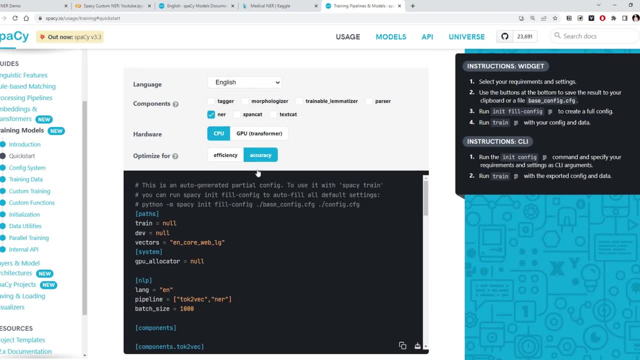 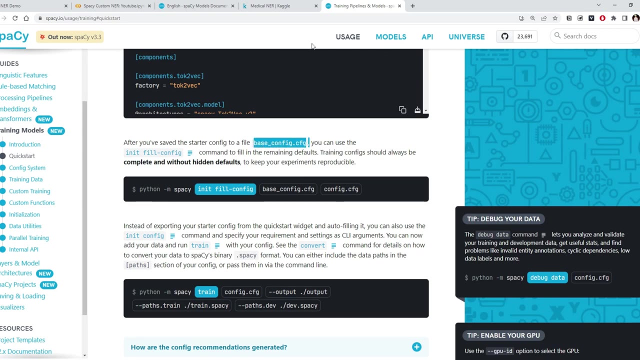 accurate model will be the larger but slower inference. but we will go with the accuracy. and then as you select, the config file gets updated. so once you select what we want, we can copy the config file and we can see we can store it as a base config dot cfg. so let's take that and clear. 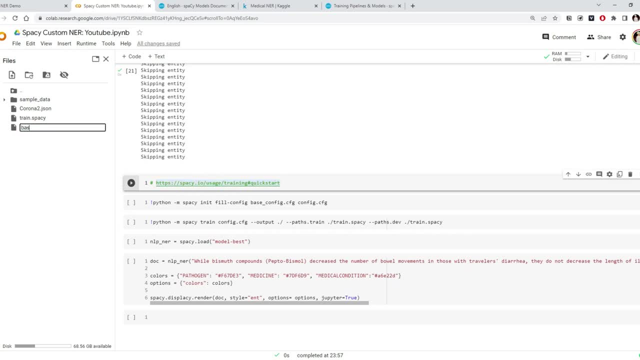 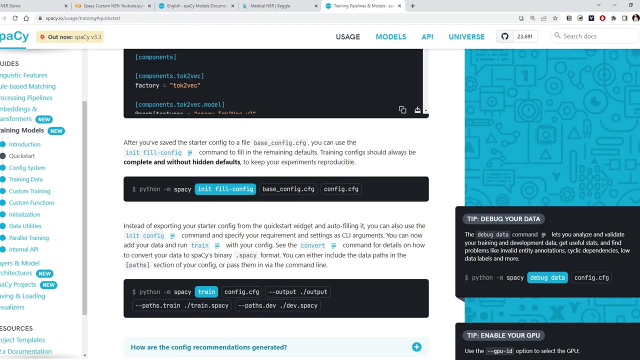 one. let's create one file here called base config, dot cfg, and we'll paste what we copied right once we created the base config, we have to run. we have to run specie init fill config. so we now we have to fill the base config and then we 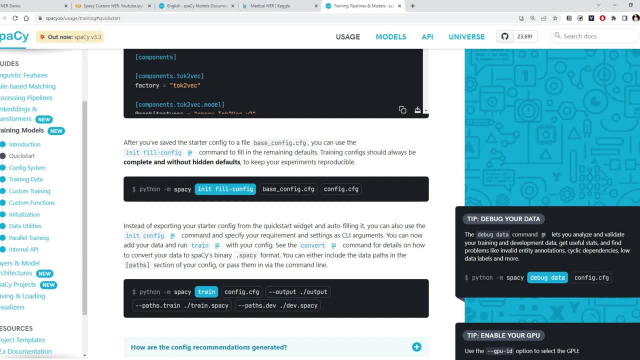 it will generate the, the final config file, so it takes our base conc strand, as per our priorities, and then it also fills some default values and finally we get the config, which contains all our selected configuration and also the default configuration. right, so let's fill this particular. 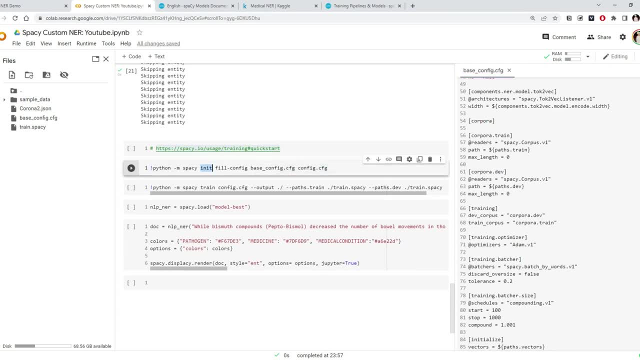 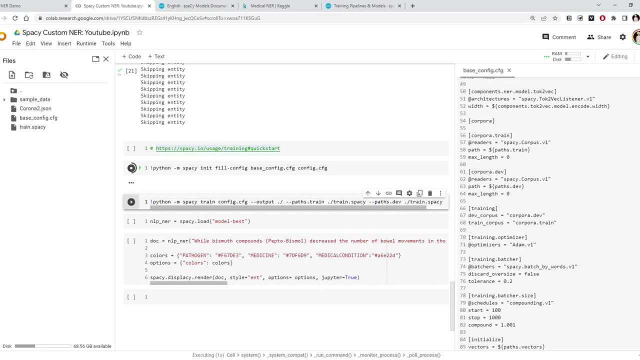 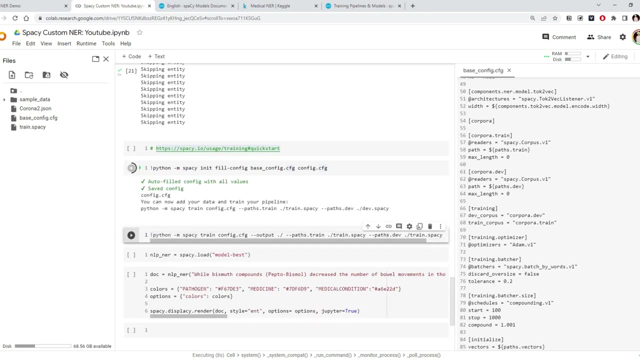 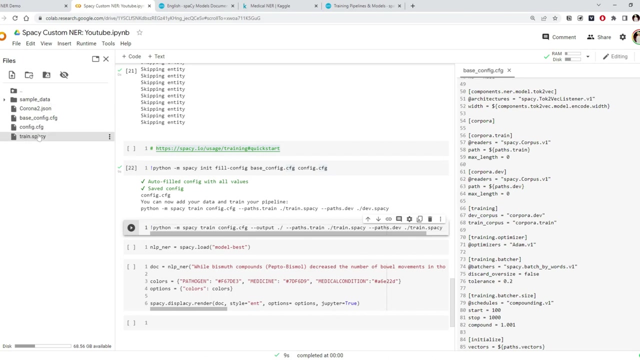 base config file. so we will run that command field config and it will take our base config and convert into the new config file. yes, it got saved at configcfg. we can see that file. yeah, and we can look at. it. has a lot of different. it has our model name, the large model name and some of the interesting thing it has. 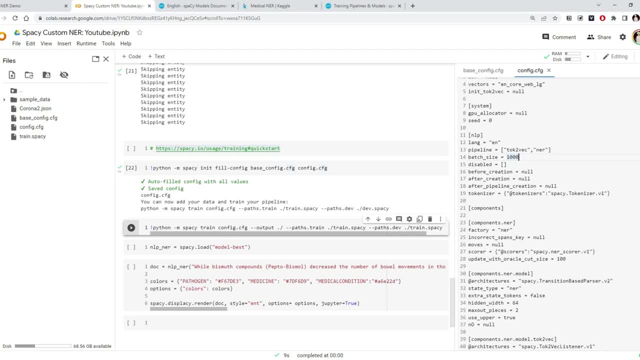 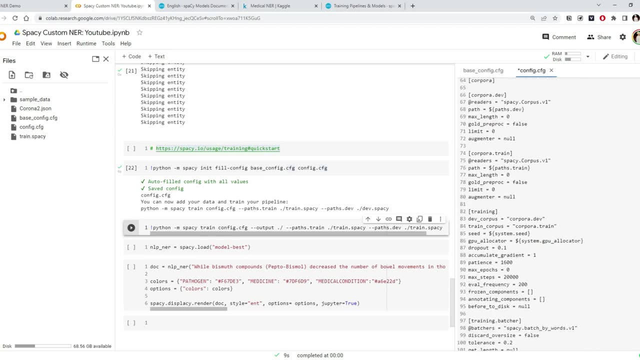 is this like? what is the batch size for training? instead of 1000, we will keep it 100. and another thing i want to modify is the training properties. if i go down, there is something called training, which is the maximum epochs for the training, and if i, if it is by default, it is zero. it will try to. 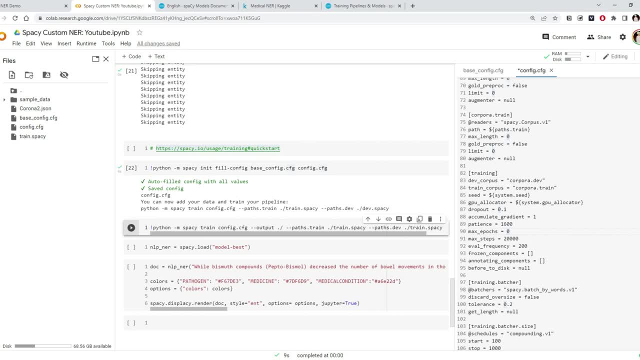 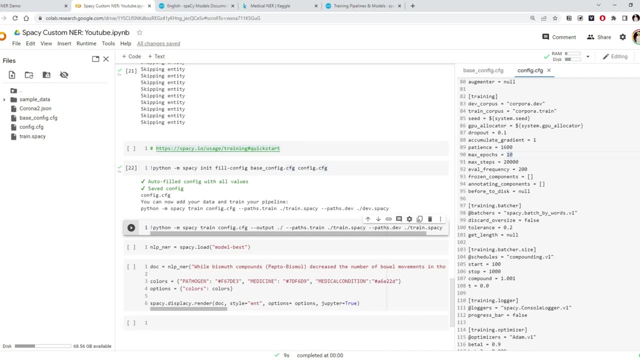 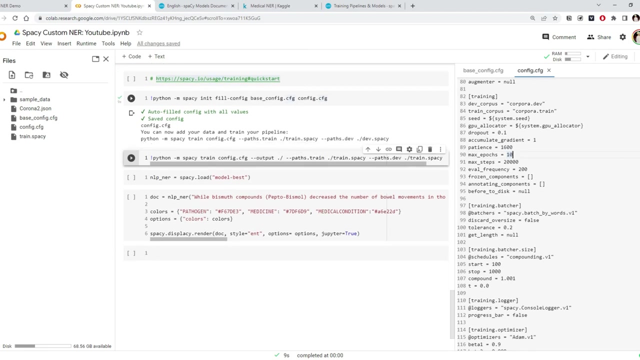 you know, optimize as much as possible, but we will only train for the 10 epochs. let's save this file. okay, now we have a config file, the final config file, and we can see: when we created the final config file, we also got the next command, that how to train our file. so we have a spacey train command, which. 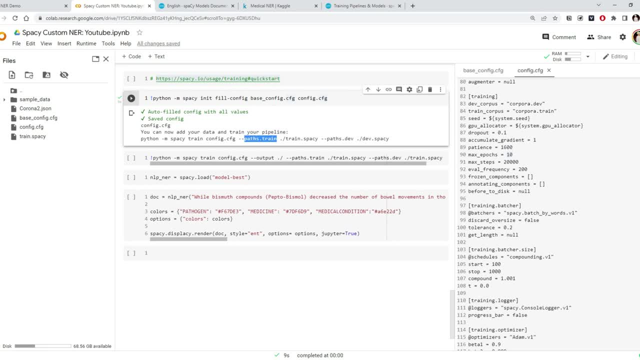 takes our config file and then we have to give the training file path and the dev or the validation path. so we have that command here. for the training path, we give the train dot spacey what we created and since we don't have any validation or the development set, we simply give. 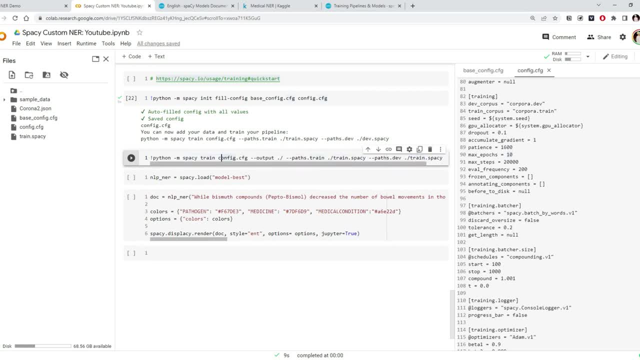 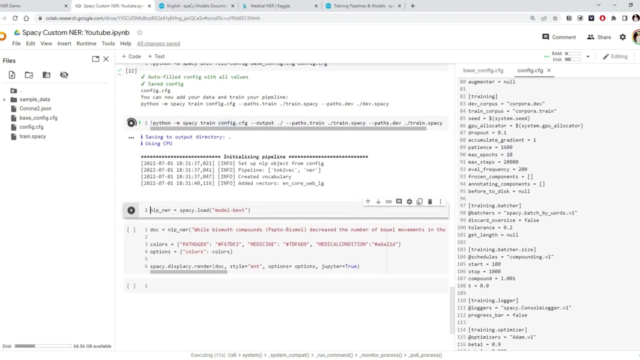 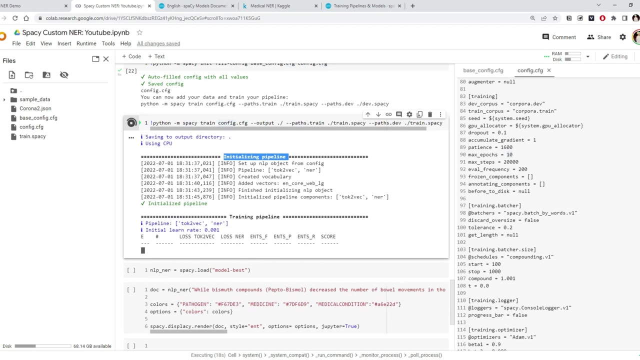 it and then train spacing. now let's run this command. it might take three to five minutes to train a spacing model. we can see some of the details, since we are running on cpu. that's what we selected during the configuration and it shows what pipeline it is initializing. it is using two. 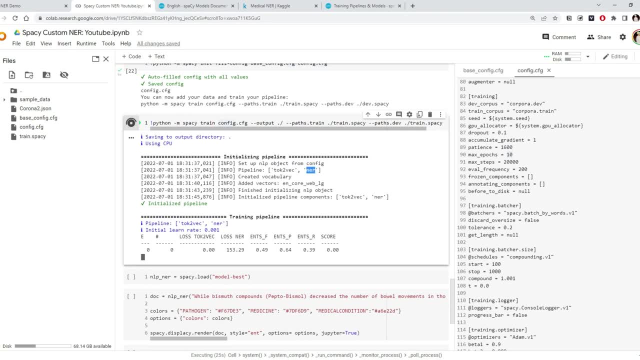 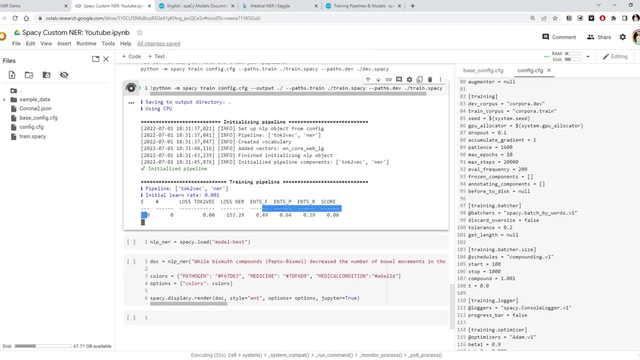 pipeline token to vector and the ner, and those vectors are coming from this model and here we can see the progress, the epochs, and we could see the loss for those, both the pipeline component, what we have, and then we have f score, precision, recall and the overall score. okay, seems to be. 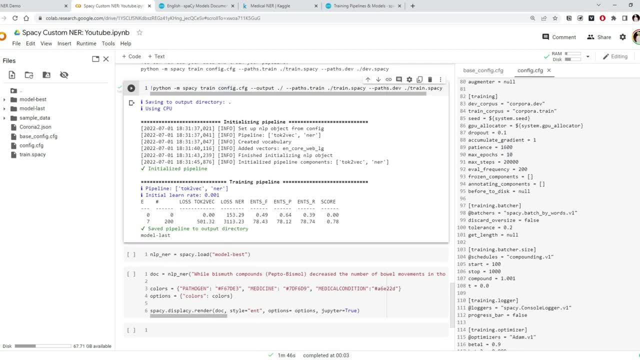 a model. training has finished because we can see here progress and model has. we can see it has saved in the output directory. if i refresh here we could see we have a model based and the model last folder got created inside the current directory, wherever we are running the. 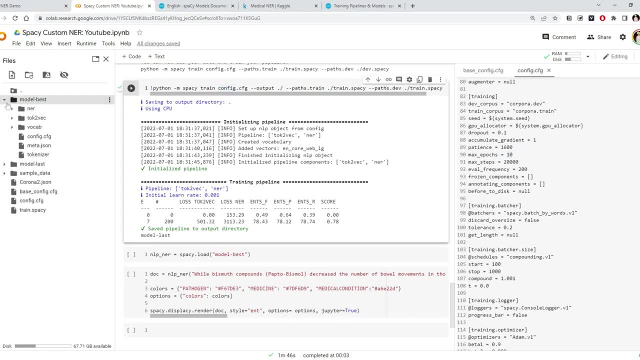 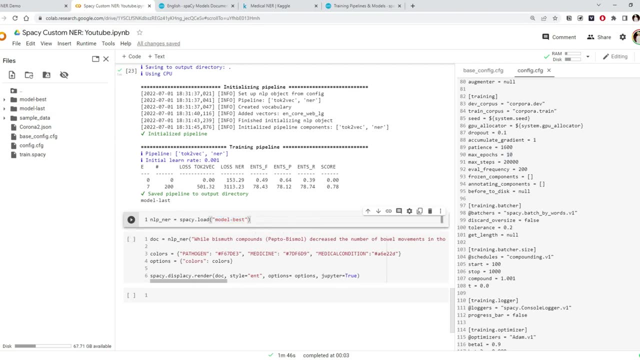 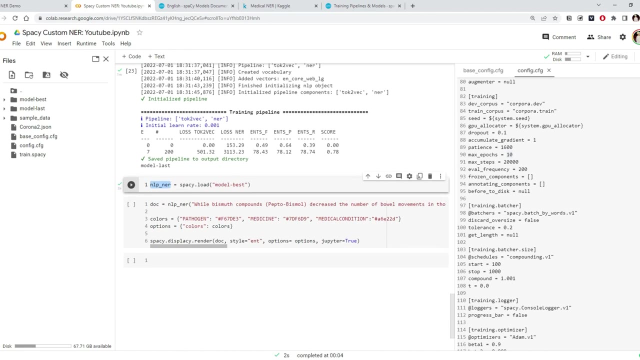 polar. we can load the model based folder. for that we have to use spaceyload. and where is our model located? we can give the model based folder path and it will load our new model. let's call that model as a nlp, nlp, ner model. once we have that model, 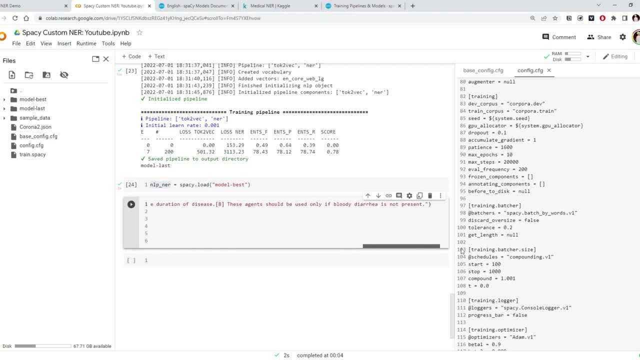 we can pass same way. that takes what we earlier for us: we are passing this medical text into it and then this time what we will do. we will also pass options, some color options, to our visualization, so we can pass our entity type. if it is pathogen, we want to use this color. 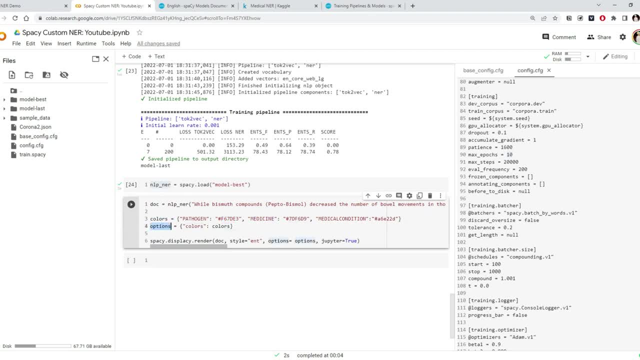 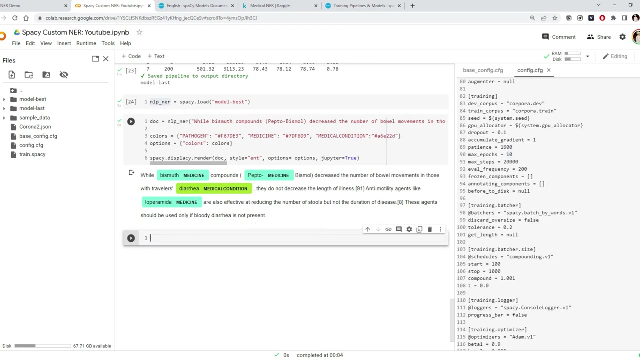 if it is medicine, we want to use this color and we can pass this color as options. so let's run the display c function again with the rendered method and pass our document, which is processed by our custom name entity recognition model, and we can see it is able to predict certain words as a custom type. now it is saying that: